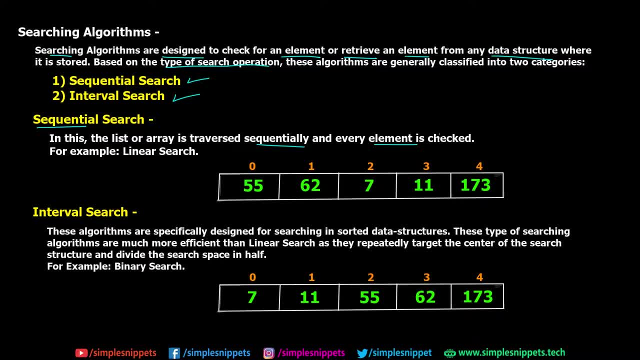 we are going to do is we are looking for a particular element in that data structure. So, as you can see right now from the diagram, we have an array data structure. We have five elements: 55,, 62,, 7,, 11, and 173.. Right, So when it comes to sequential search, let's. 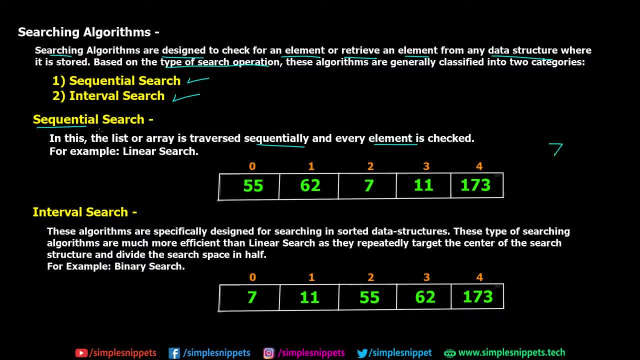 say we want to search for the element seven. so in sequential search what we will do is we will start off from one end of the array. So let's say we are starting off with the zero index, we will access this position. we will check if 7 equal to 55, it is not equal, right then? 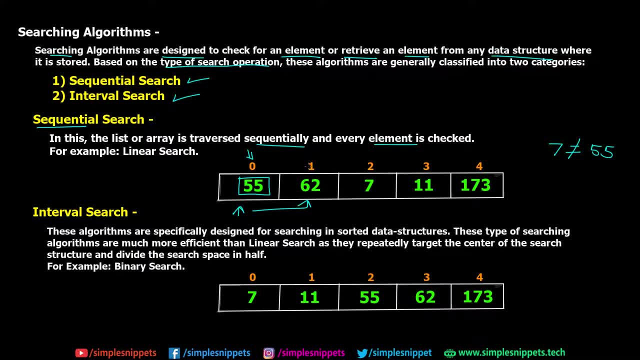 we will move on to the next element. so now we are accessing the second element. we will check whether 7 equal to 62. it's not equal right- then we will move on to the next one and at the third location we are getting 7 equal to 7, and once we find that element, we 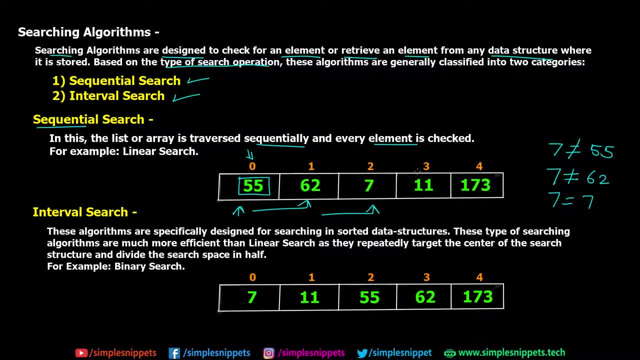 will print the appropriate message. and in case we do not find that element at all, let's see we are searching for some random number, 73. now, 73 is not there in the list, right? so we will traverse the entire array starting from one end. we can also start from the index. 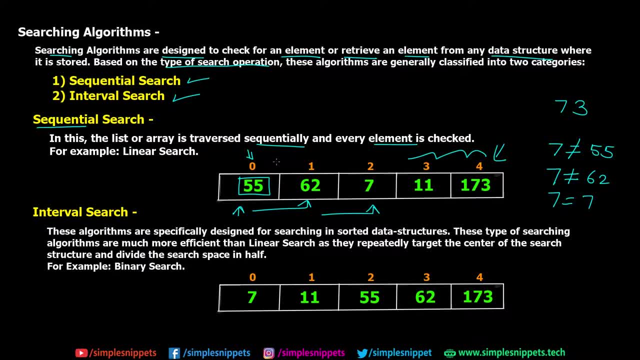 position 4 and move on backwards. it's gone. it's not gonna have any effect. but once we completely traverse it and do not find the match, we will print a message that we did not find that element. so this is basically sequential search and it is not really efficient. 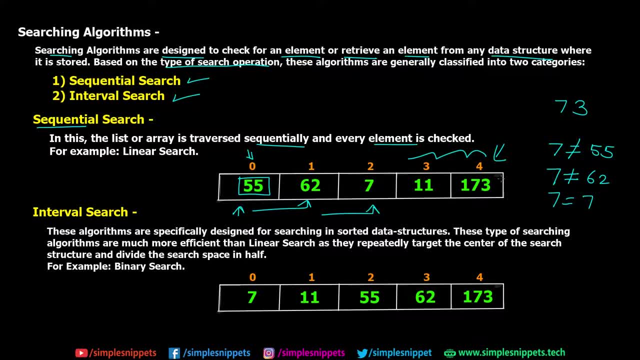 enough, because you can see, as the number of elements in the array or list would increase, the iterations will also increase, right? let's say we have an array of 100 elements and the element that we want is at the end, and if we start from the 0th element, then we will. 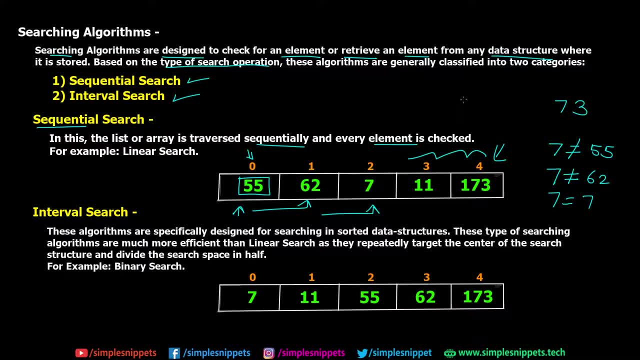 have to traverse 99 times till we reach our final output or final element right. so it becomes time consuming when the number of elements increase and it's not really used all the times. the example of sequential search is actually linear search, so we are gonna be looking at linear search today. the other type is interval search. we will discuss in. 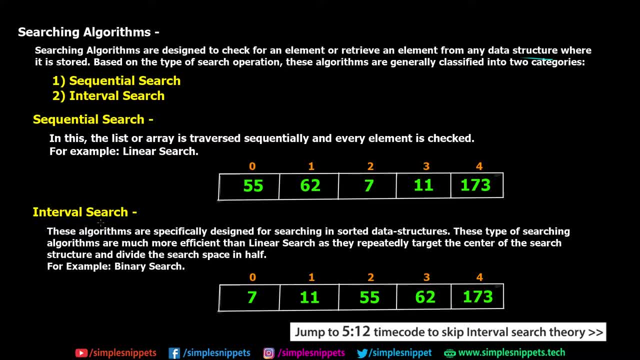 detail different types of interval search algorithms also as we move ahead. but essentially what it does is, unlike sequential search, these algorithms usually work on sorted data structures. So here you can see the same array, but here the numbers are sorted in ascending order. we have 7, then we have 11, 55, 62 and 173. in ascending order, in the increasing order right. 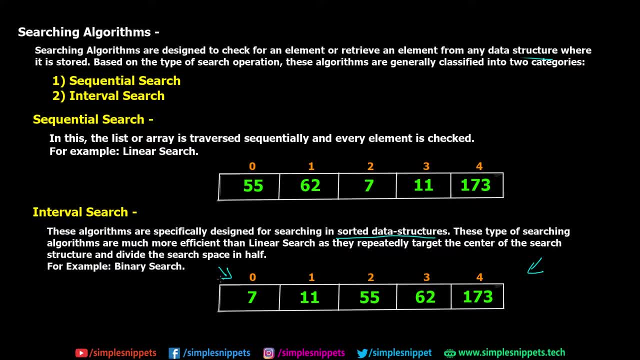 So these interval search algorithms specifically work on such arrays or data structures only when in the elements are ordered in a particular fashion. and these type of algorithms are much more efficient than linear search as they repeatedly target the center of the structure and divide the search space in half, or essentially they do not traverse every element, you know. 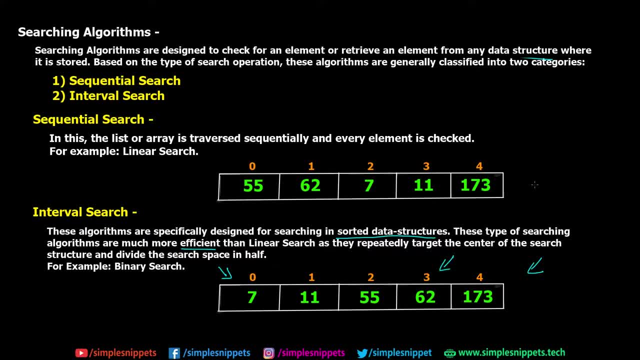 let's say you want to search for 62. 62 is over here, right? So an example of interval search would be binary search, and what this algorithm does is it divides the array in half every time and searches in that half array. So if you want to know how to do this, then you need to know how to do this. 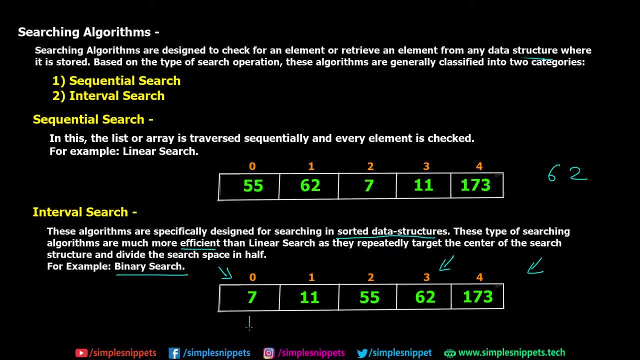 So if you want to know how to do this, then you need to know how to do this. So, for the first time, what would happen is just to give you a small example. this would be the first part of the array and this would be the second part of the array. 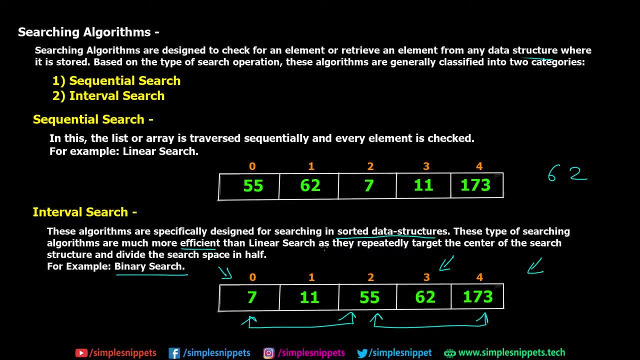 So in the first step, what will happen? we will have two subarrays and since this is arranged in a particular order, in ascending order, we can check the starting and the ending position right. So this is the start element S1 and end element E1 for this subarray. and this is the start. 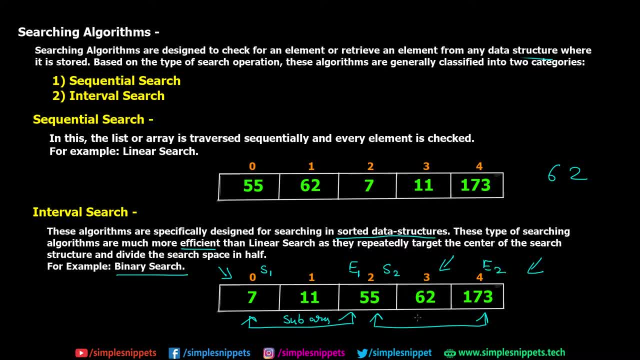 element, and this is the end element For this second subarray right. So we can check these individual values and we know that 62 is greater than 55. So once we know this, we know that 62 is not present in this subarray right. 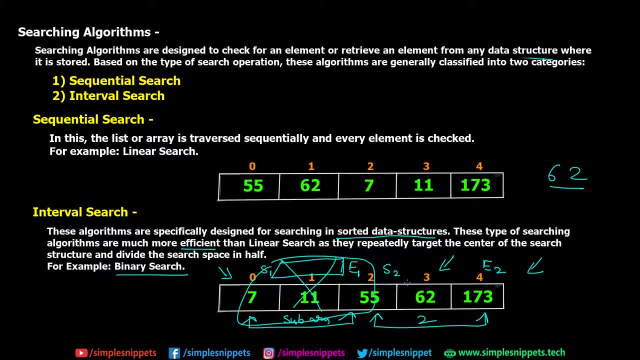 So we will not search in this entire subarray, we will directly search in this subarray and then the process will go on till we actually reach our output or element. Of course we will discuss this in detail- binary search- in the next video or in upcoming videos. 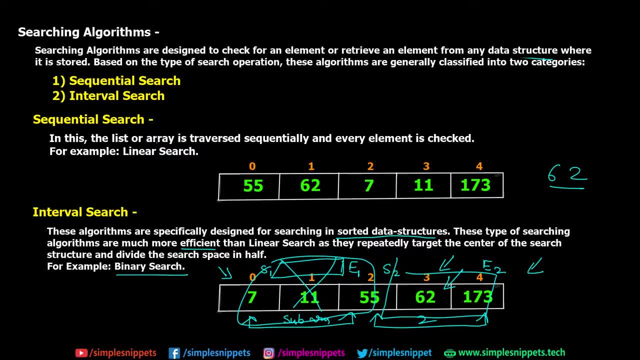 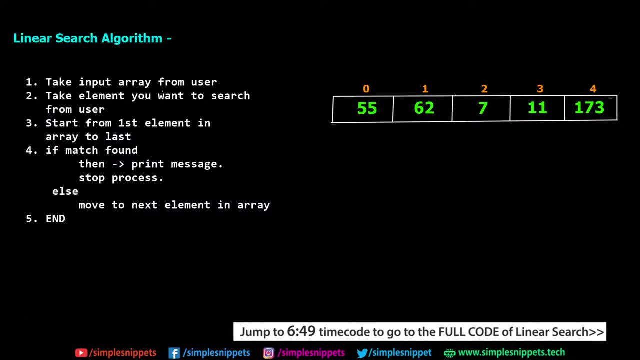 Right now let's just focus on sequential search. So let's see in detail a type of sequential search, that is, linear search algorithm. Okay, so in linear search what we do is we take the input array. So we are going to be applying linear search on array data structure. for simplicity purpose, 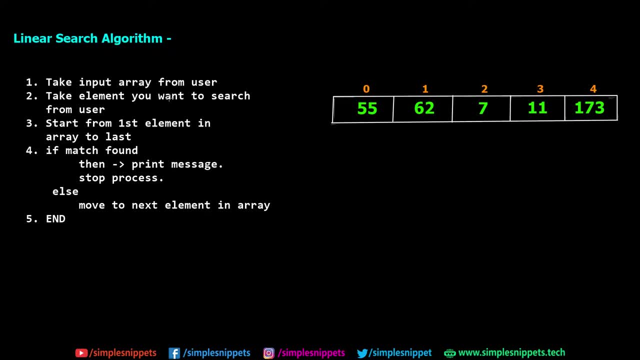 but linear search can also work on linked, linked list or queue or stack, wherever there is a sequential way of storing data, you know. So the step number one is take input array from user. So let's assume this is the input array that the user has entered. 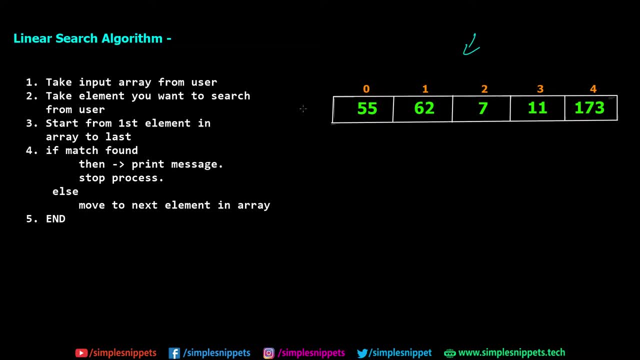 We have five elements and they are not really in any order, So linear search can work on unordered list also. The second step is take elements you want to search. So let's say user wants to search a value of 11. okay, So we'll start from the first element of the array to the last. 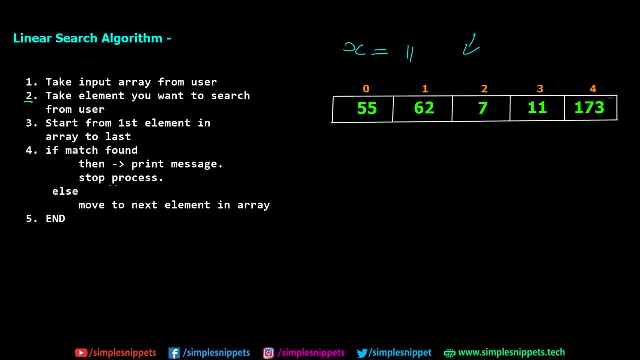 You can also go in reverse order. If match found, then print the message and stop the process, else move to the next element in the array. So this is a very basic algorithm which is written in pseudocode kind of language, and we will also see the programming part. 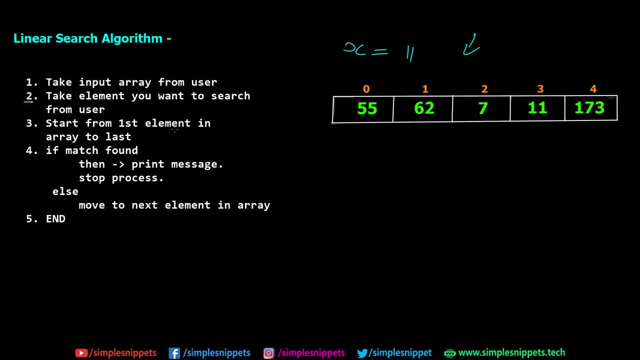 We will convert this algorithm into C++ programming and implement this search algorithm also, But we will first start. we will go to the first element: check if 11 equal to 55, no right, then we will move on to the next and then we will move on to the next and this step. 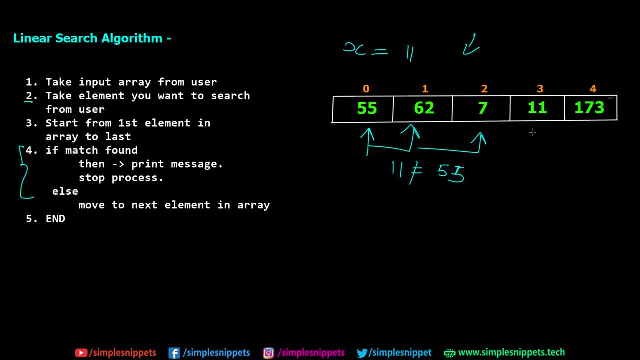 number four will keep on executing till we find the match. So once we find the match, we will just print a message that match found. and if we traverse the entire array and do not find a match, we will just print a message that we did not find that particular element. 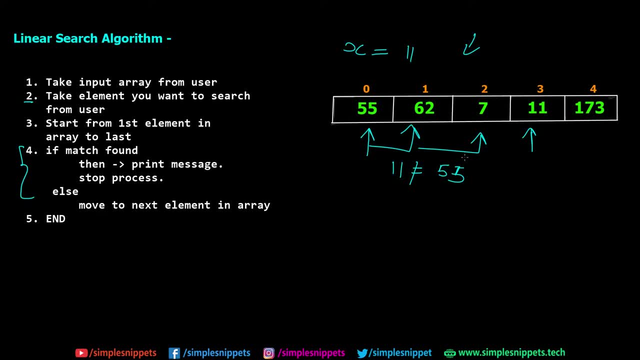 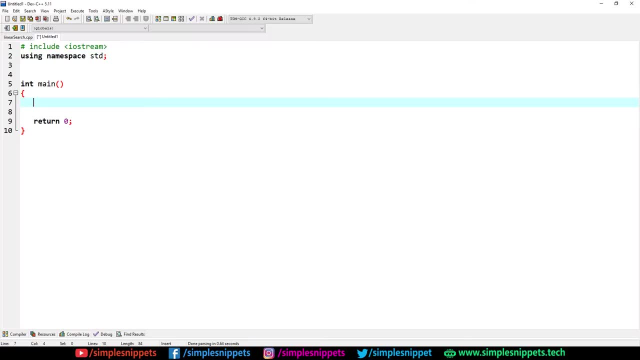 Okay, So this is a very basic linear search algorithm and let's go ahead and quickly implement this in a C++ program so that both theory and practical will be covered. Okay, so, as you can see on the screen, I have my basic C++ programming structure and I'm 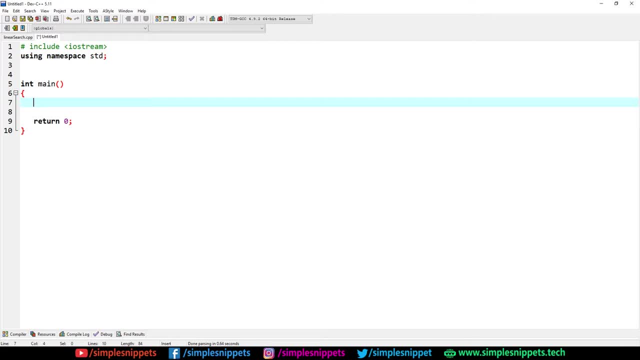 using Dave C++. you can also use any other ID. you just need to know the algorithm, and then the syntax is the only thing that matters. In fact, if you are using any other programming language, even that will do- Java, Python or any other general purpose programming language- but we are going to be using C++ programming. 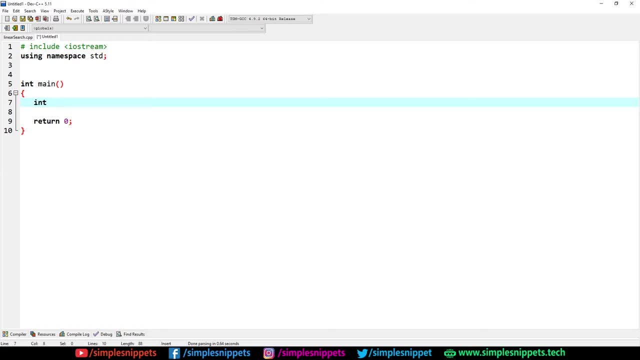 So let's get started. let's create an array. for simplicity purpose, we will hard code the values. now what we will do is we will ask the user: please enter an element to search. now, remember we are using an integer array. it can also be of any other data type. it can. 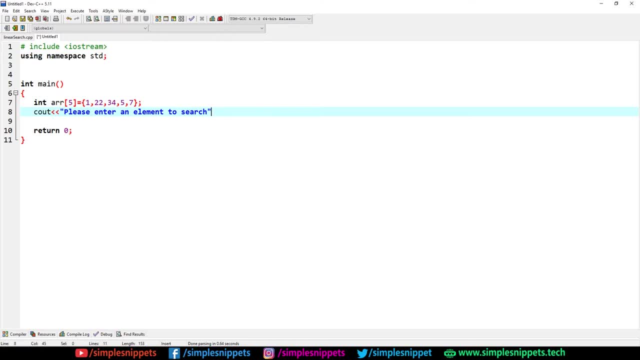 be double float. in fact, it can even be a complex data type. if you're using classes or if you're creating a user defined class, I'm going to say int num. okay, we will take this integer from user and what we will do is: let's create a user defined function over here. I hope you. 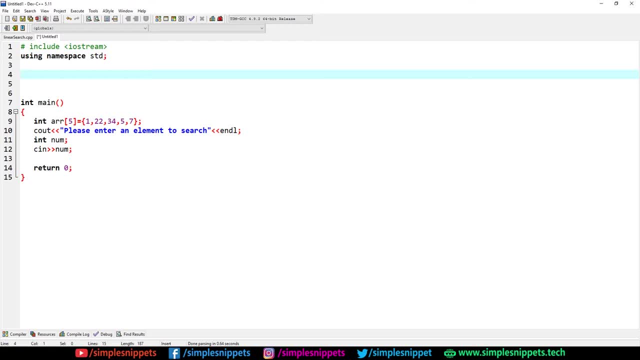 know the concept of functions. I have a complete C++ tutorial playlist. if you're confused, you can go check that entire playlist out. I'll drop the link in the video description. so I'm going to say: void: Linear search. okay, inside this we will pass an integer array and we will also pass the. 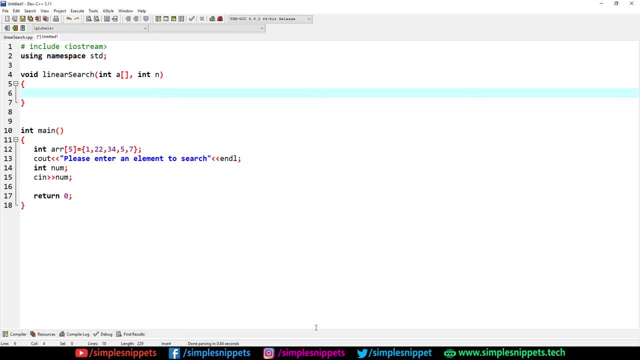 number that the user passes. okay. so whatever number we are taking here as num, we will pass it over here. we will say: linear search, arr, comma, num. okay, so we are passing arguments in this user defined function that we are creating over here. it accepts an array, so 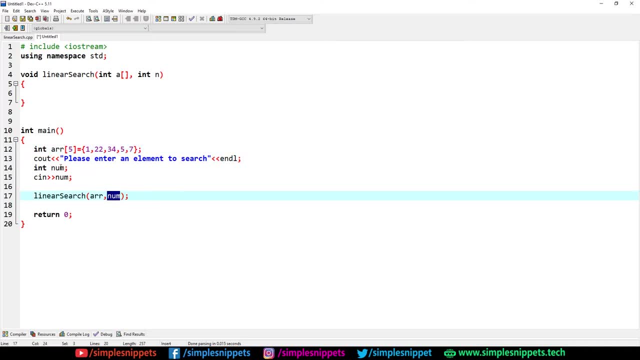 this is how you pass an array: array as argument And this is the number that we're taking in from the user which you want to search in this array. Okay, so now the real implementation, or the real algorithm, will be working, or will be implemented inside this function. So let's do that. So first, 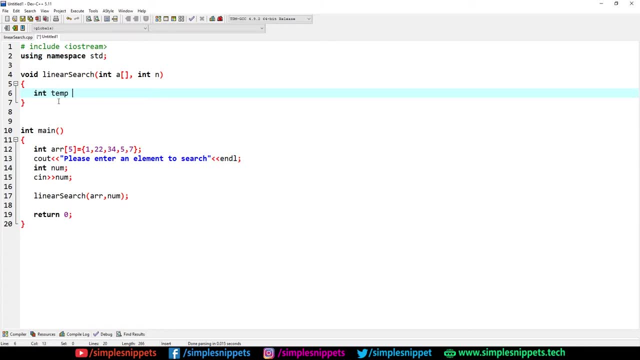 things. first, we will create a temporary variable in temp equals to minus one and assign minus one to it. I'll tell you why we do that. Next thing, what we'll do is we'll say: for int, i equals to zero, i less than five and I plus plus. Now, since we've hardcoded the size of 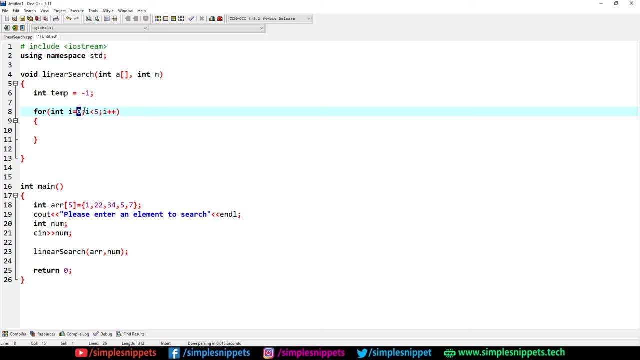 the array and we know that the size of the array is five. we are going to loop through the entire array, right? we have to search each and every element. So we will start from zero index and we will go till four array index starts from zero to four Right. So 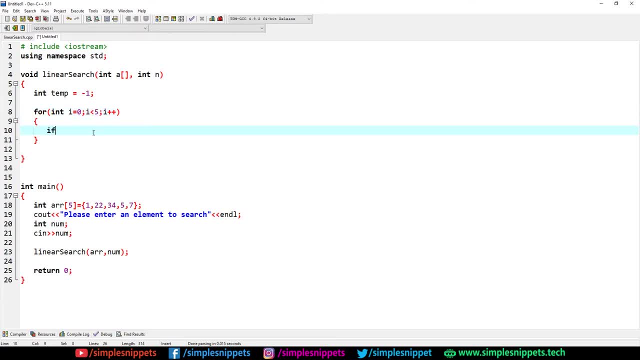 that's why is less than five. Now your. if we say if a of i equal equal to n, so n is the number that is num that we pass over here in argument. so if we get a match, let's print out a message element found at location colon and we will print out this: I, which is a iterator. 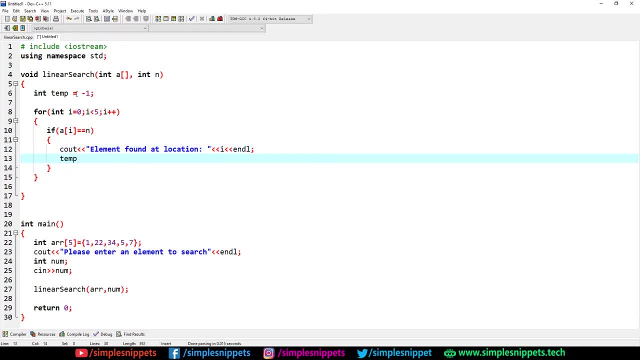 and it will give us the current position right. and here we will also make temp equals to 0. okay, I'll tell you why we are using this temp. now, when we come outside the for, we will just check if temp equal, equal to minus 1, and here what we will do is we will simply 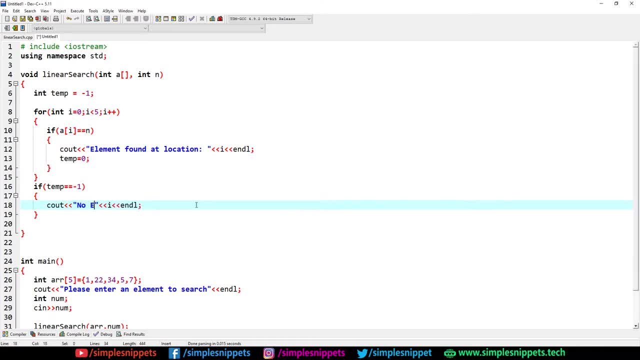 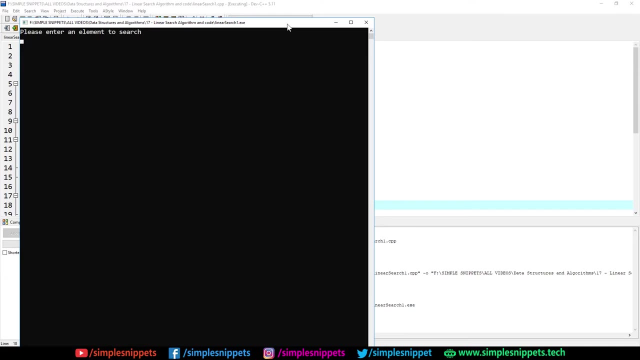 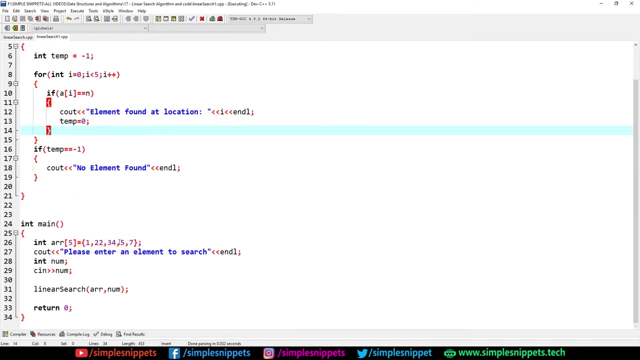 say cout: no element found. okay, now let's try to save this. I'll say linear search: 1. okay, and let's try to compile and run this. Okay, so our program is working fine. it's saying: please enter a element to search. now we've hardcoded the values of the array, which is 1, 22, 34, 5 and 7, so let's enter 7 over here. 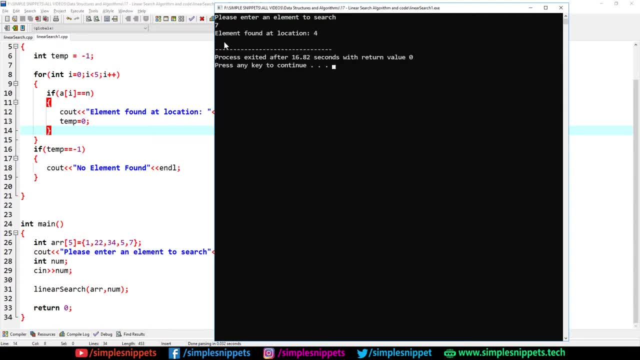 and let's see if you are getting an output. if I hit enter. so there you go. you can see element found at location 4. location 4 is the last index value, right, so 0, 1, 2, 3 and 4. let's try to execute it one more time. compile and run. 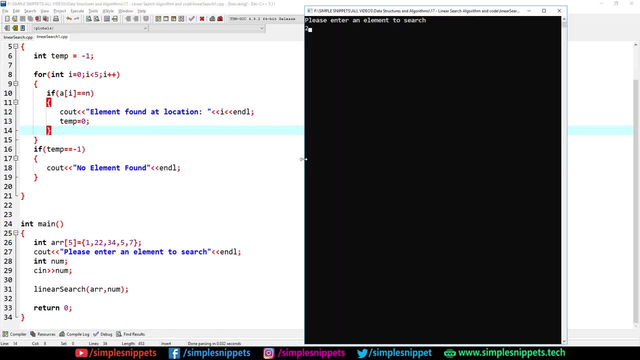 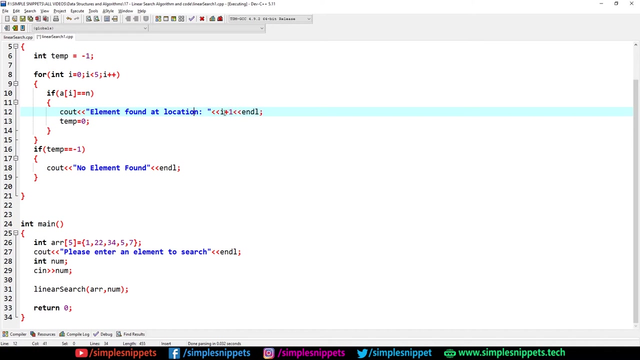 Now, this time I'm gonna enter 22, just to cross check if our code is working fine. and there you go. element found at location 1. location 1 is basically second position, right? so 0 index over here, and then 1 index is of 22. if you want, you can also do a plus 1 over here, and 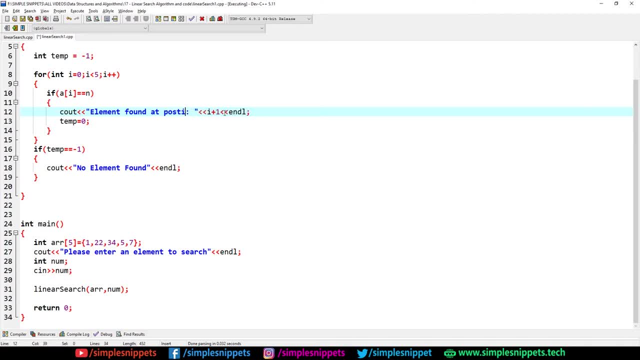 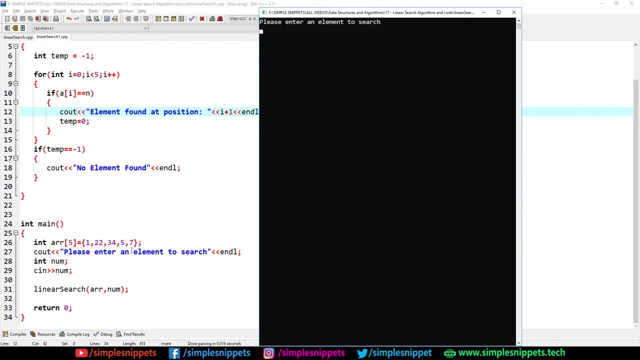 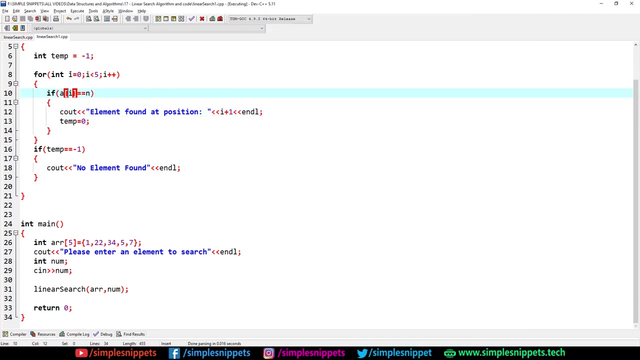 you can say at position: Just save this, compile and run. now, if I'm searching for 34, I should be getting an output of position 3. so if I say 34, hit enter element found at position 3, so it's at index position 2, but I'm adding 1 over here, okay, and we are getting a match over here. so that's why we. 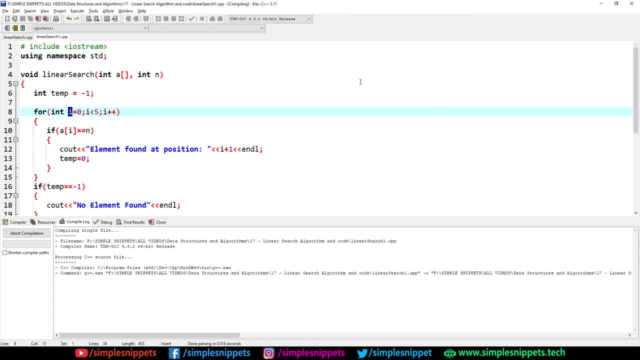 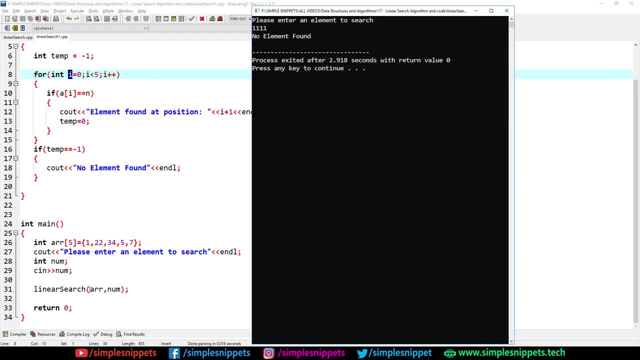 are printing the i value, let's enter a wrong number. let's say it is 111. if I hit enter, no element found. So what was happening is In the code. We are passing this array, which is hard coded values, and we are passing the number, so right. 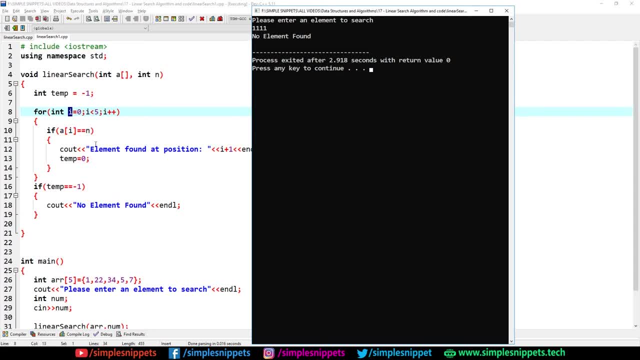 now we passed 111, 111, right? so in the function, what happened in the for loop? we started from 0 and we went till 4. in every iteration we are checking if a of i- that is, for the first time a of 0 equal, equal to n. a of 0, we know, is 1. 1 is not equal to 4 times 1, right so? 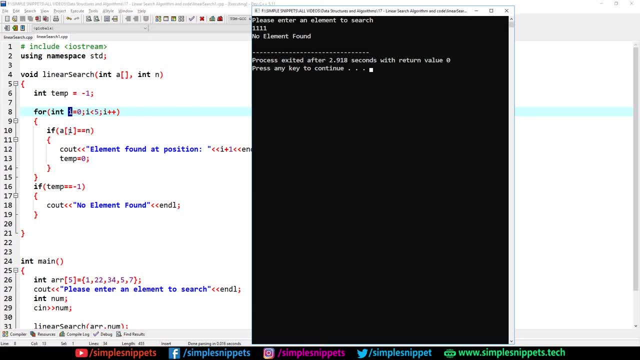 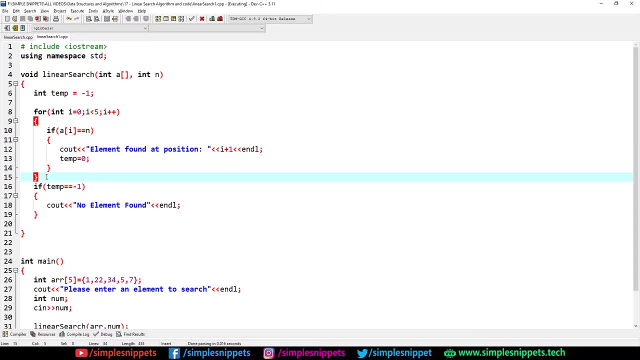 this: if block will never be executed, even for the second iteration the condition is checked. so basically this: if block was never executed And we never made, temp equals to 0. so when we come outside this for loop over here, we are simply checking if temp equals to minus 1. initially we assigned temp equals to minus. 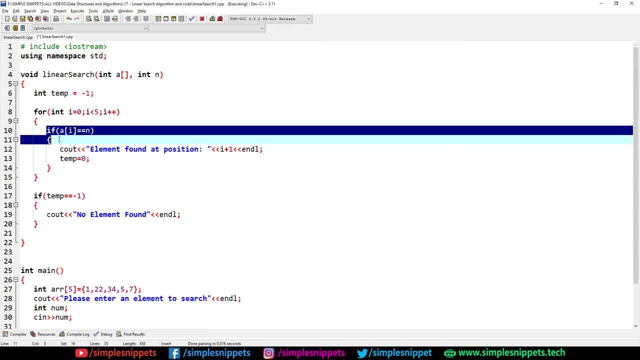 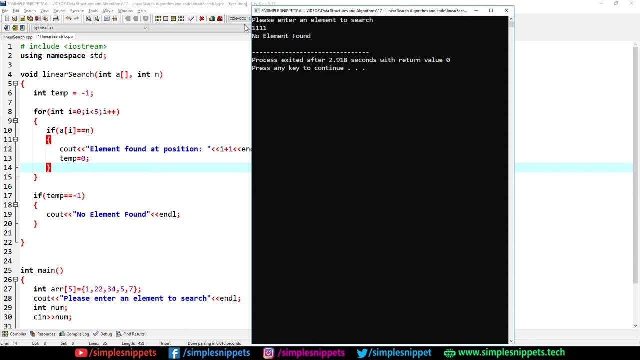 1 and it did not get changed because we never got inside this if block right. so at the end also, temp is equal to minus 1 and that is why now we know that, since this if block never got executed, the value of double one, double one that we entered, is not matching anywhere. 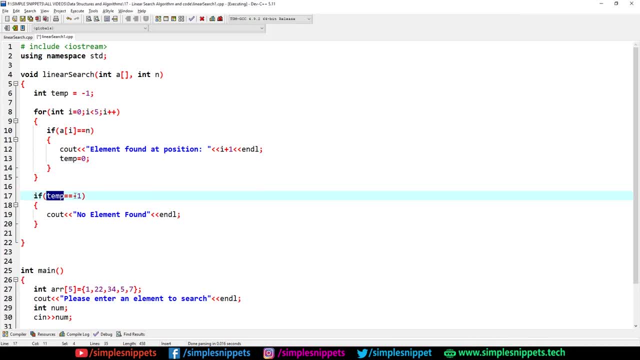 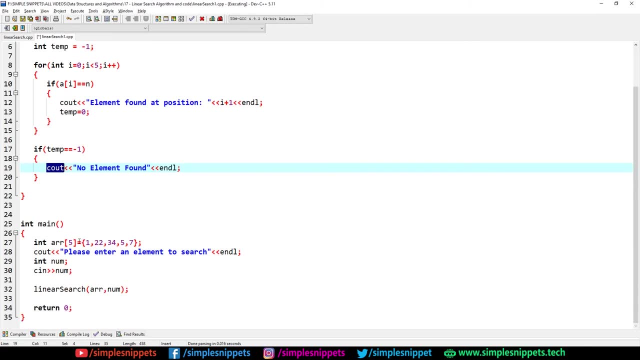 in the entire array. So now that's why this- if temp equal equal to minus 1 is true, and now we can print no element form. okay, so this was a very simple implementation. what you can do is you can also take this array from the user, right? so if you want, you can just create this array. 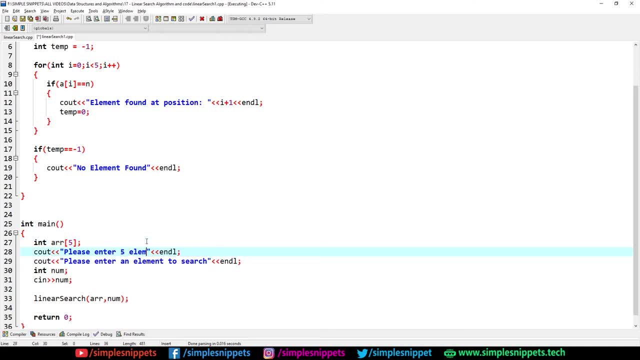 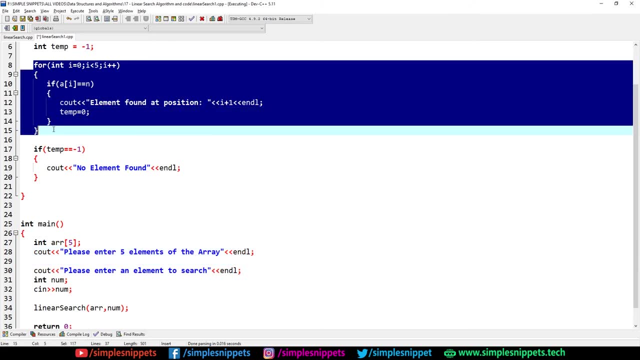 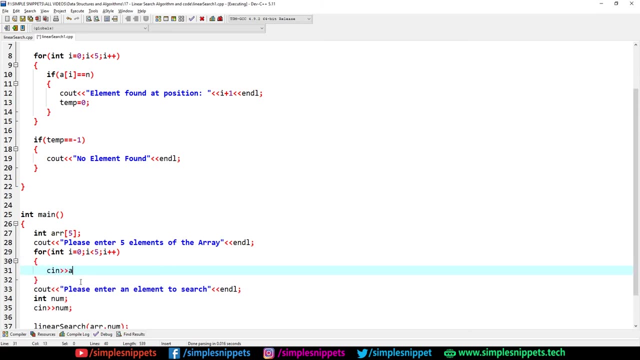 and you can print a message. please enter five elements of the array. okay, now you can use a for loop again. I'm going to copy paste this Inside the for loop. what you can do is you can say c in arr of i, so at every iteration. 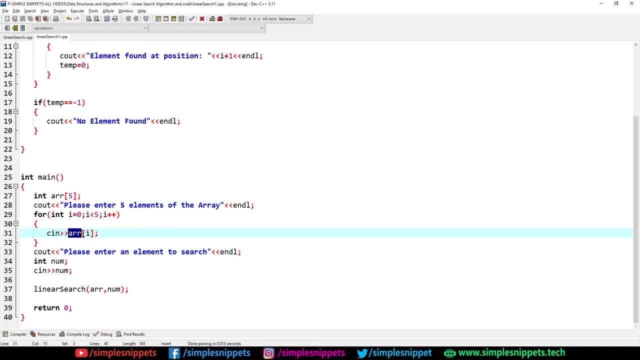 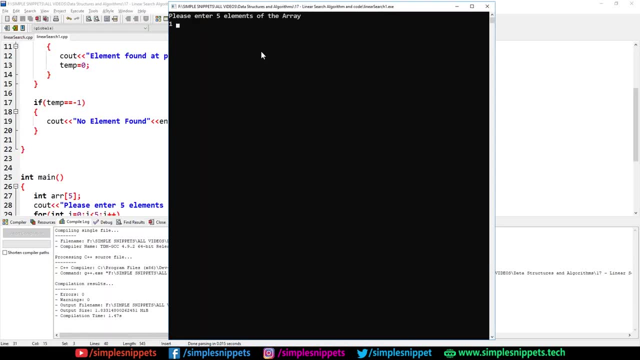 you take input from the user. let's save this and let's see if this works. I'm going to say compile and run, okay, so it's now saying please enter five elements of the array. so I'm going to say 1, 45, 54, 66, 73. if I hit enter now it is asking please enter an element to search.